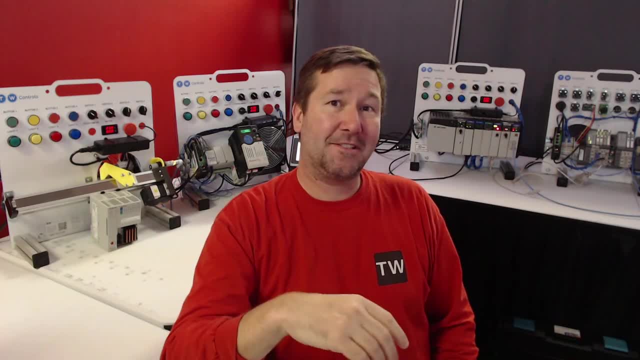 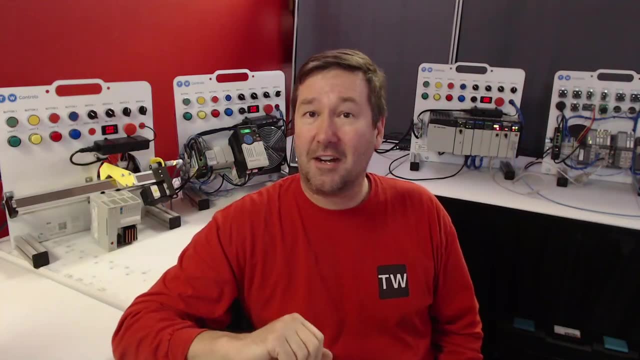 I upset some engineers today. They were wanting some training for their technicians and I always ask: what is their current experience and where do you want them to get to You? give me those two points and I'll tell you if our training is for you or not. And they wanted online training. I. 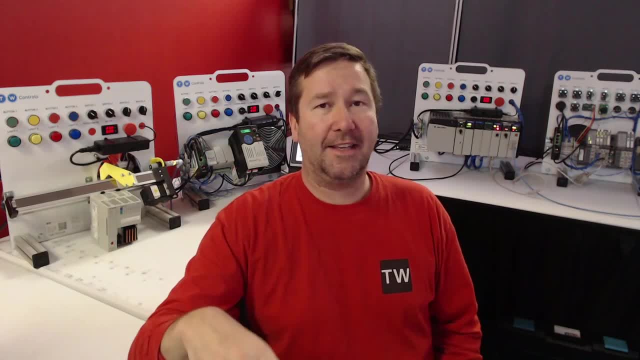 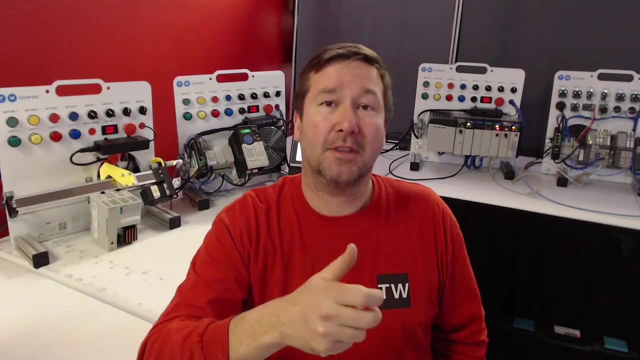 told them right away you can't teach troubleshooting online, And they said we just need them to understand enough to identify the components and then we'll FaceTime with them and they can point the phone at it and we'll do the troubleshooting. I told them you didn't give them any better. 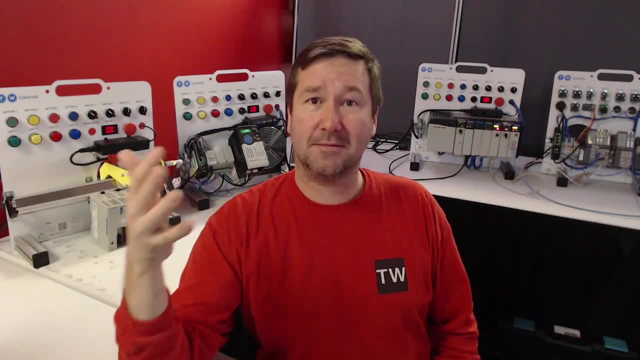 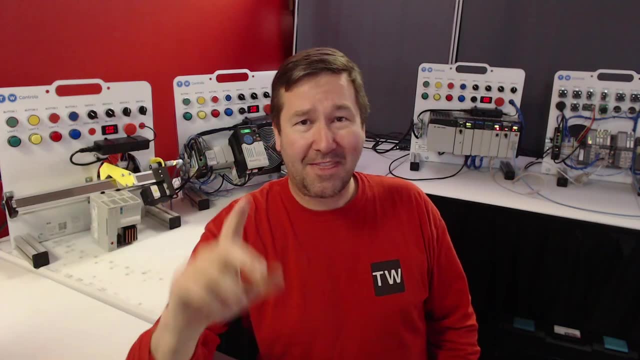 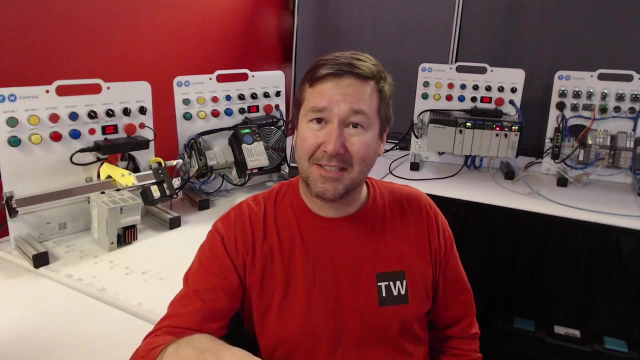 troubleshooting skills. You turned them into a very expensive cell phone holder. That ended our discussion about them coming to our class, but I thought it opened the door for a very important discussion that I have been wanting to have, And I'm going to try to use a story to tell you about. 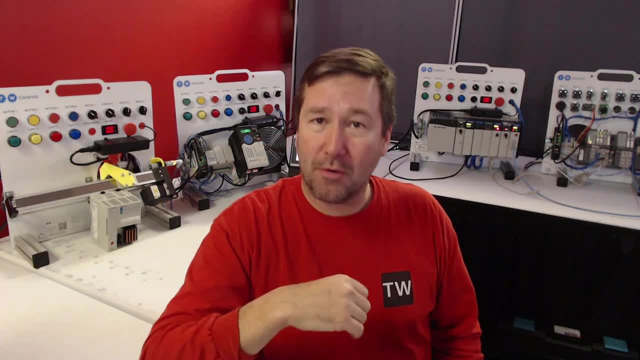 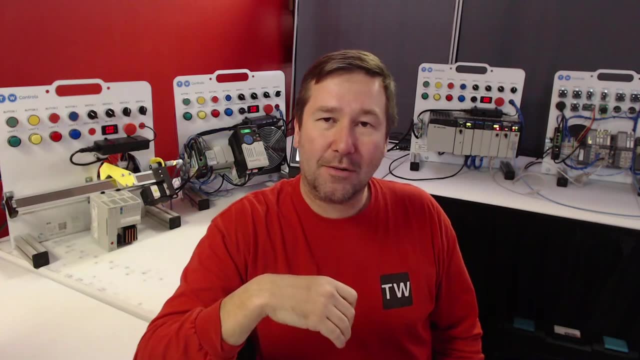 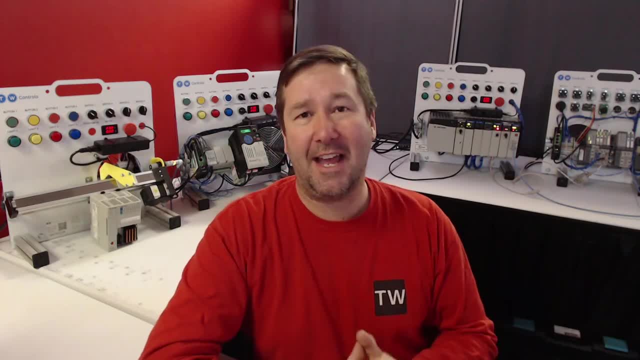 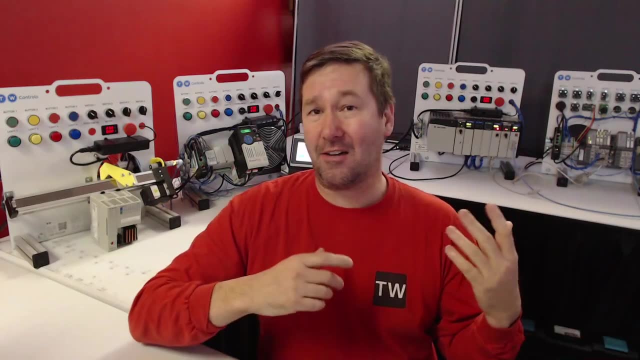 braking systems there are, And Engineering Ed has not only designed that braking system so that it can stop the car as fast as it can start the car, he has also designed it so that it can deal with the heat stress of you constantly hitting the brakes and letting off the brakes, hitting the 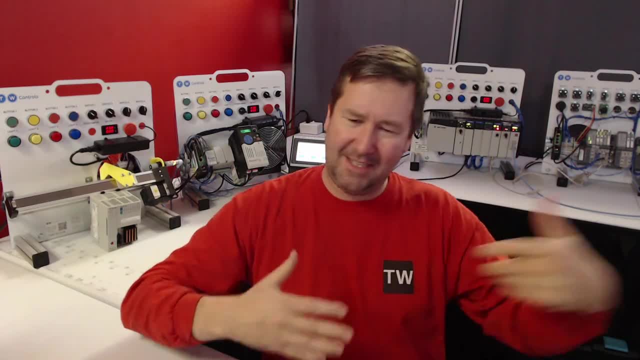 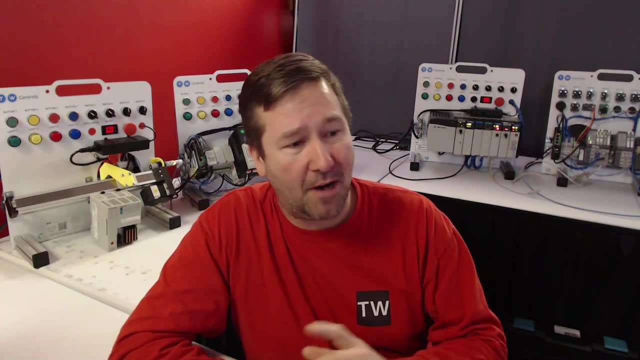 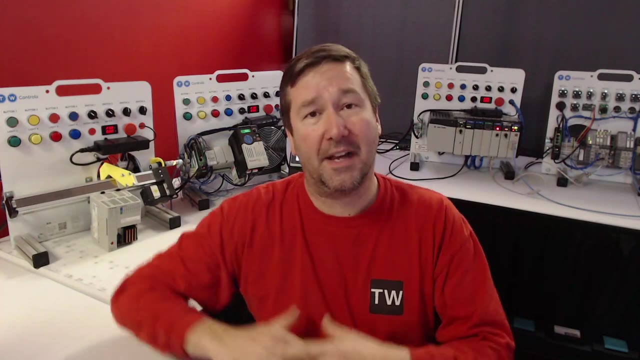 brakes, let off the brakes, He's cross-drilled the rotors and he has ducked the air, and he has made this an engineering marvel. Not only that, but he understands manufacturing processes, So he has designed it so that Assembly Al can easily put this on. Assembly Al has a robot that does most of the assembly for him. 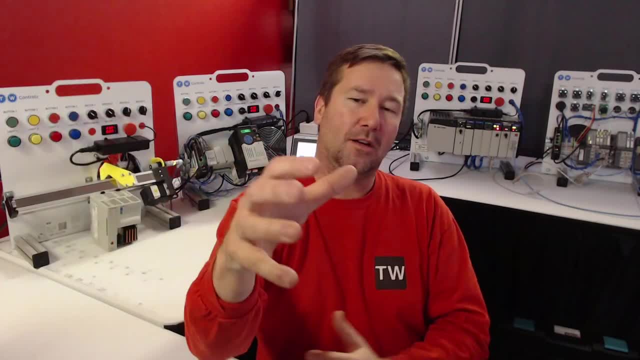 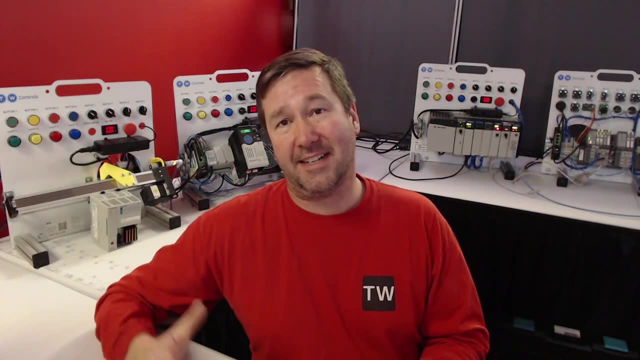 and all he has to do is grab that caliper assembly, slide it over the rotor and put two bolts in. It is an engineering marvel, even on the assembly line. Now, technician Tim, he's never seen an assembly line before and he doesn't understand why. Engineering Ed designed a car. 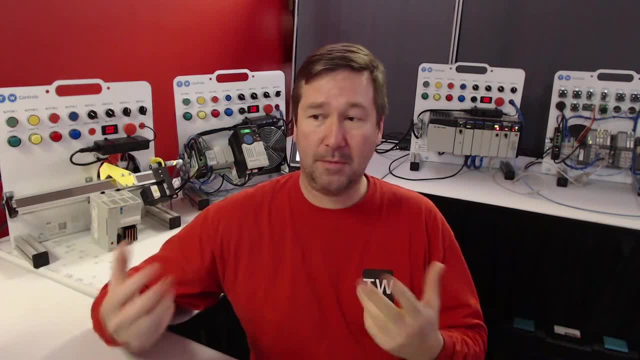 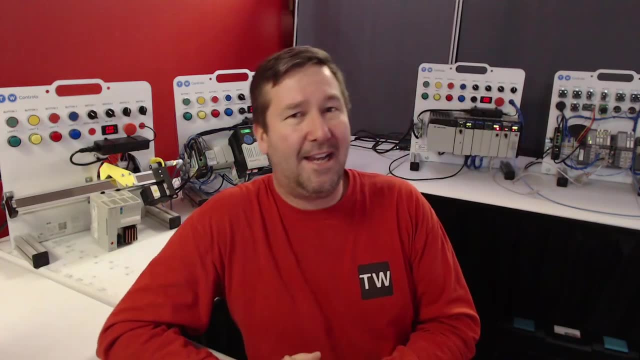 that in order to inspect the brakes, you have to raise the car up, remove the tire and remove the inner fender well, and kind of have your head cocked sideways. But he knows that's what he has to do. Now this leads me to my grand question: If your brakes are grinding, which one of these three?